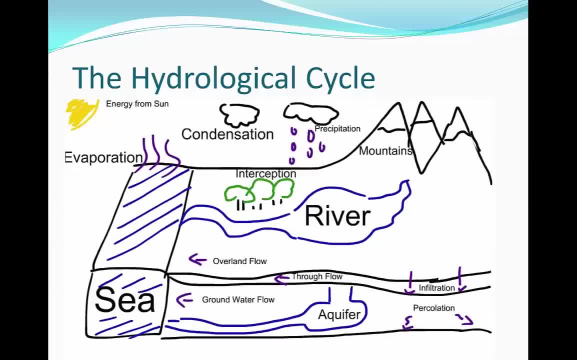 The Hydrological Cycle. This is a diagram of what you have to know for the Hydrological Cycle in AS, Human Geography. Now it's also known as the Water Cycle, and the Water Cycle is something that's been studied in the early years of education. 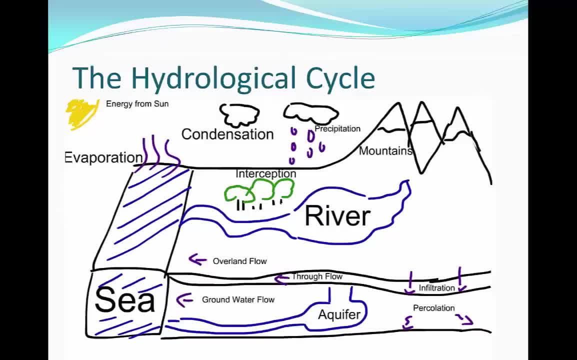 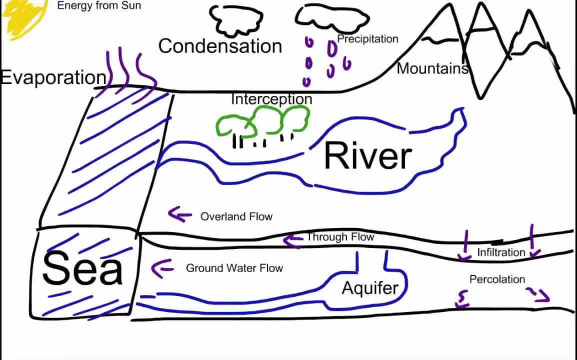 So this is a lot more in depth and contains all the information that you have to know, So I'm going to go over it now. So here I've drawn what it should look like at our AS level. So, as always, we always start here at the sun. 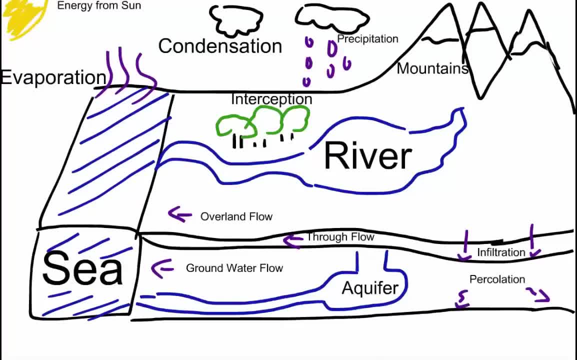 So we begin at the sun, and that's where we get our energy from. So, now that we have energy, we then begin to evaporate the water in the sea. Now you're not going to have to know all the terms and processes. 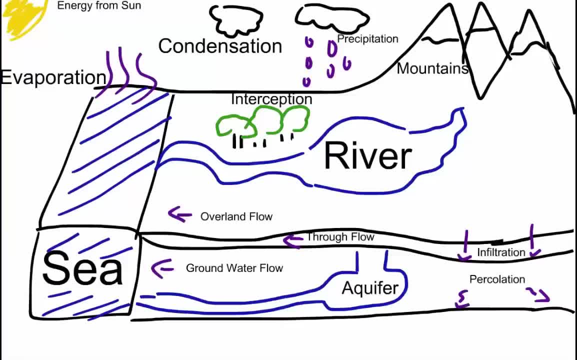 As well as you may have to have done in, for example, GCSE Physics. All you have to know is that evaporation is when high temperatures turn liquid drops into gaseous molecules. So once we do have these liquid drops here in the sea right here turn into gaseous molecules. 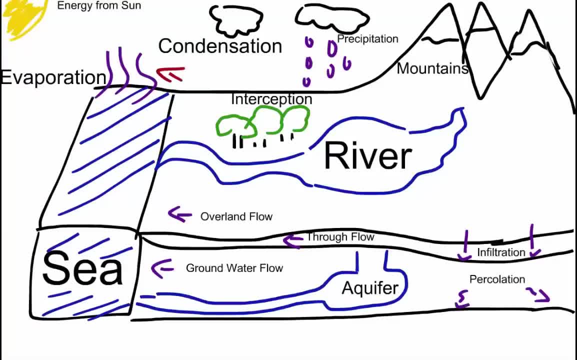 they move up, as shown here by the evaporation streams of water vapour, and then they condense. So what happens in condensation is that the cool temperatures then turn gaseous molecules into liquid drops again, So then it turns into this cloud. 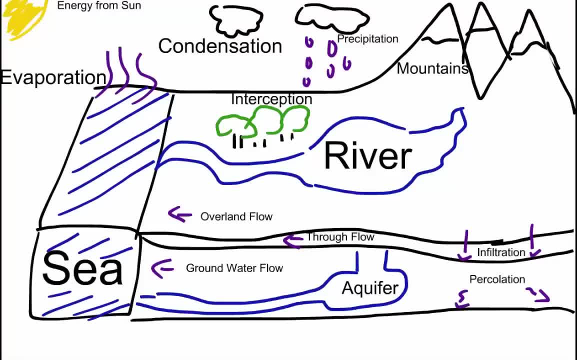 Once a cloud then gains a lot of mass and it's not able to support itself, the liquid drops then fall to the surface, formed in a saturated atmosphere, And then the saturated atmosphere must be sort of quite high up, just above the mountains. 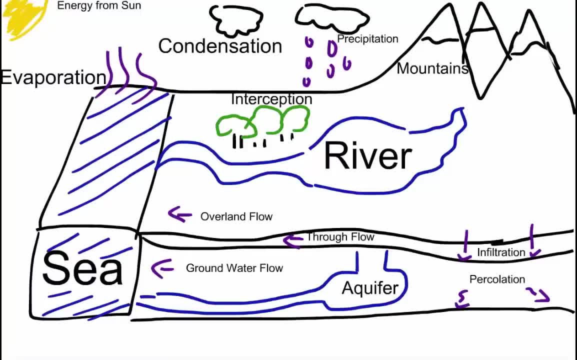 Of course, this isn't drawn to scale, it's just drawn to make it easy to the eye. So now that we've got our water drops falling, a lot of them drop here on top of the snowy mountains, Some drop straight back into the sea. 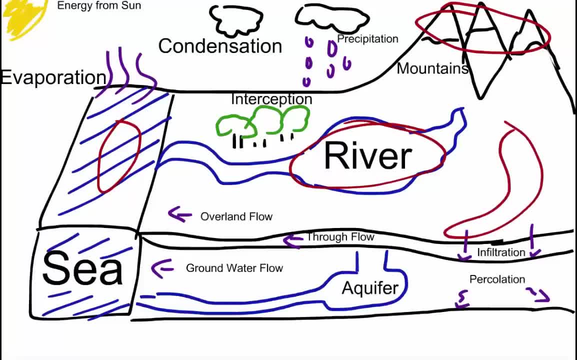 Others into rivers and then the rest here just onto the land. So it drops everywhere and then the water from the mountains, of course, then evaporates on the snow caps and then it moves down here into the river. Once it moves into the river, it can then stay in this store here, which is a lake. 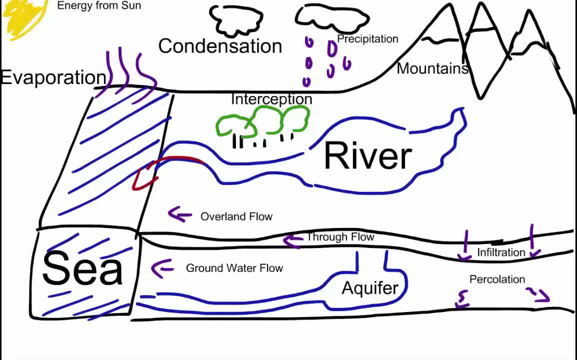 and then moves all across back into the sea, where the cycle can then begin again. However, some of the water is intercepted here by the vegetation. What that means is that the vegetation then gets the water and is storing it, you know, for whichever purposes the plants may need it for. 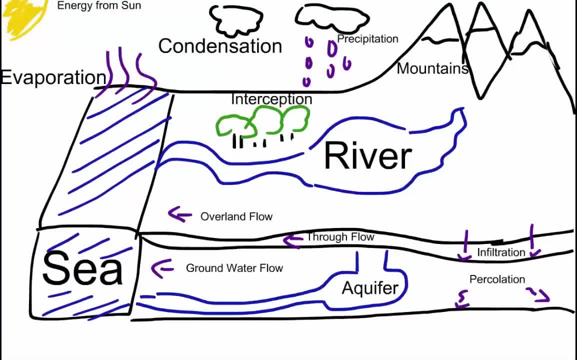 Now there is a thing called stem flow, where the water moves through the vegetation towards the sea, but that's not something that's going to concern us at the moment. Then, for the water that lands on the land, there is overland flow. 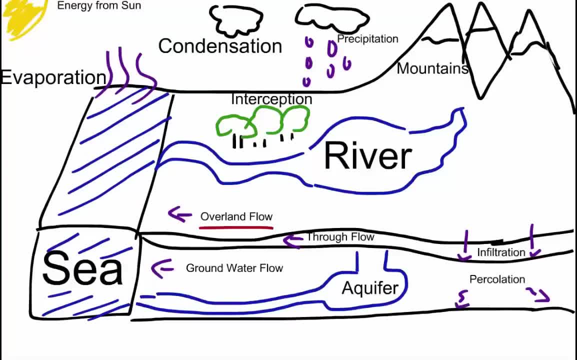 which basically means that the water just moves down across the sort of face of the land back into the sea directly. Okay, now you've probably seen this layer here which I've drawn on, where there's a little break between the overland and then the, where you know underwater is the bedrock. 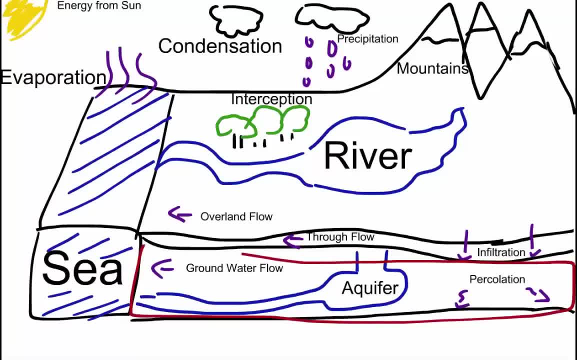 So this layer here is known as bedrock. If you're copying the diagram, I'd probably advise you to write that on there in case you forget. But this little layer here is the layer of ground that separates them both. This is pretty much the soil right here. 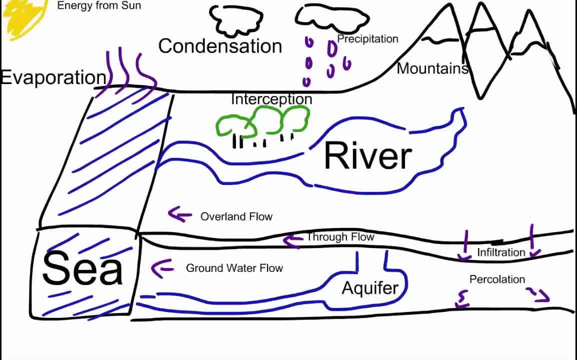 So in the soil we have a thing called through flow, where the water doesn't quite go all the way down to the bedrock, but it then does travel towards the sea. But how does the water get from the overland down to the soil? 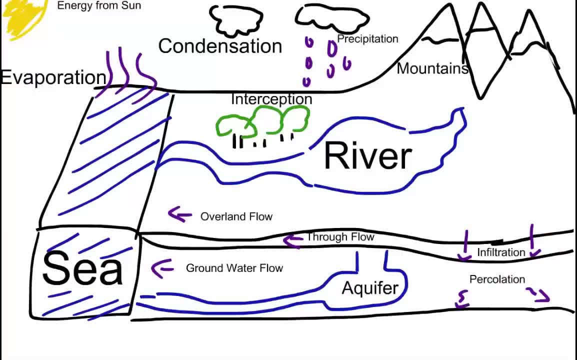 And that is infiltration. So infiltration is the absorption and downward movement of water from the surface towards the soil And then, once it's in the soil, it can then percolate, which is the vertical movement of water down the bedrock. 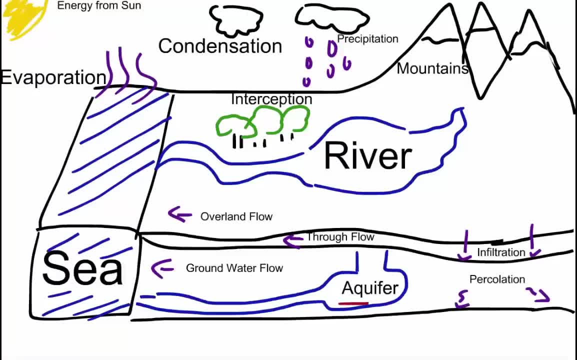 So percolation is that, And then what causes the water to reach this aquifer over here, which is an underground store, And then that enables the water to travel out and go towards the sea. So, in summary, we have a lot of ways in which the water can actually reach the sea. 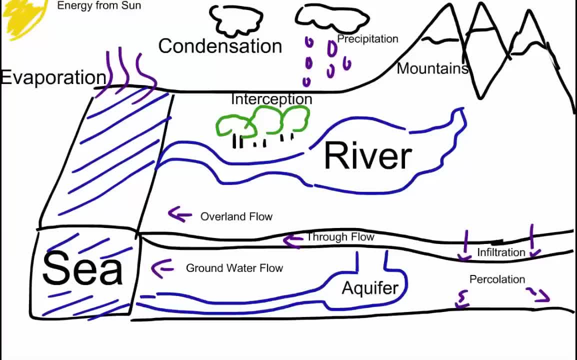 whether it be precipitating back onto it or overland flow, groundwater flow down with the river. There are really tons and tons of ways. So right now, I'd like you to copy this, If you haven't done so already. go over your notes. 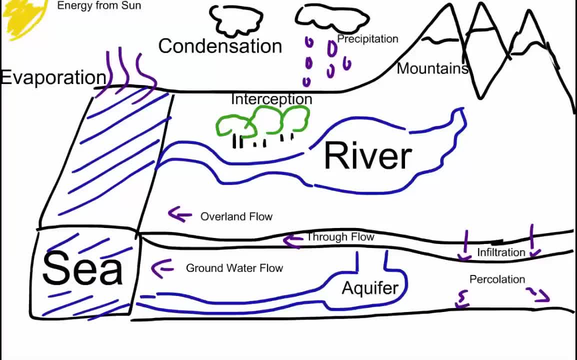 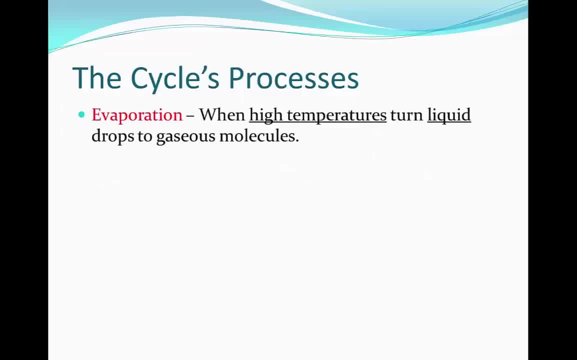 and then we're going to look at the definitions of the processes. Okay, now that we've gone over how the hydrological cycle works, we're going to look at its processes. Evaporation: This is received from the energy of the sun.